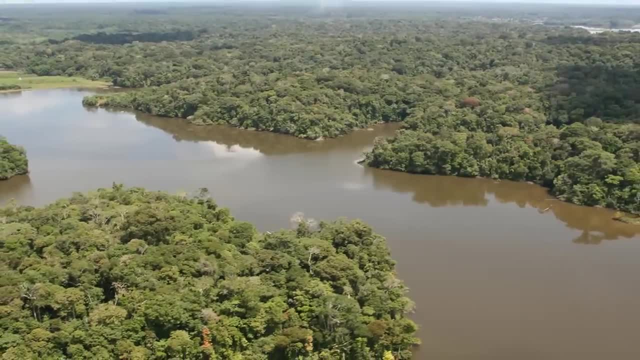 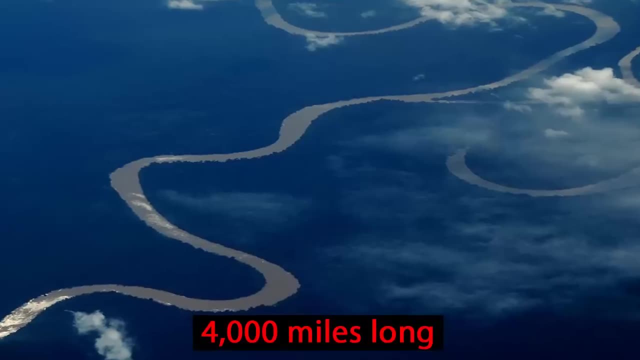 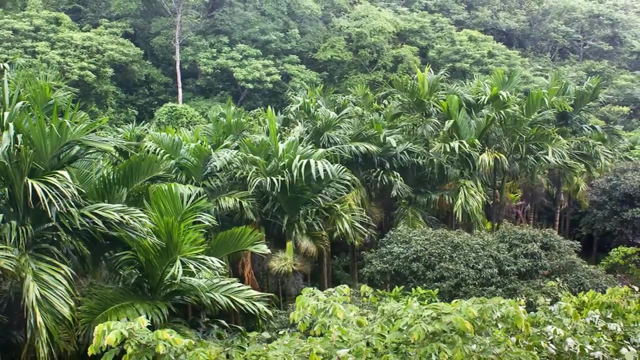 You will also hear this rainforest called Amazonia because the mighty Amazon River runs through it. The Amazon is 4,000 miles long and is the second longest river in the world. As their name tells us, rainforests get much more rain than anywhere else in the world. It usually rains about 260 inches each year, but can reach as much as 400 inches. Not only is it wet, it is also very warm. since it's so close to the equator. The average daily temperature is usually between 86 and 95 degrees. 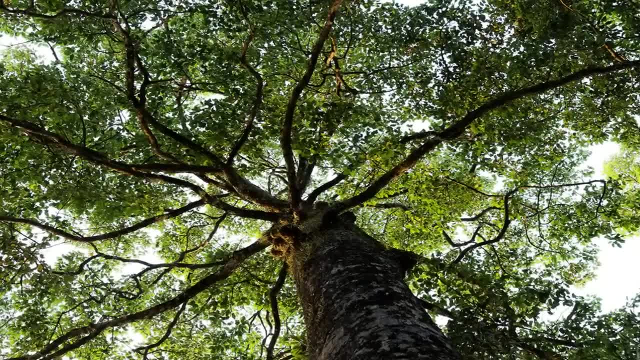 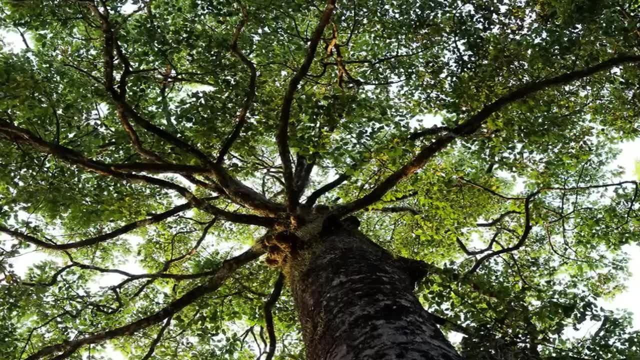 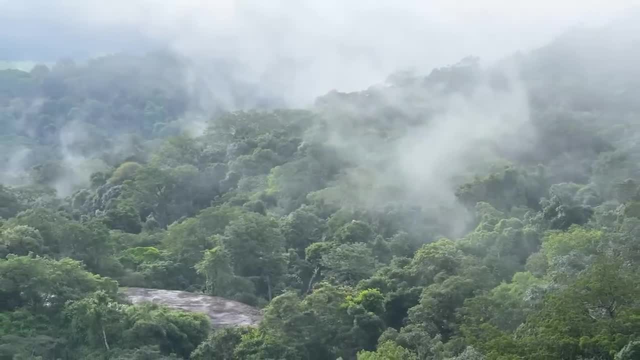 A wet and warm region like this means that everything grows well. This explains why the trees are so incredibly tall. Some parts of the rainforest are in mountainous areas. Up high, the treetops are always covered in a rainy, wet mist. 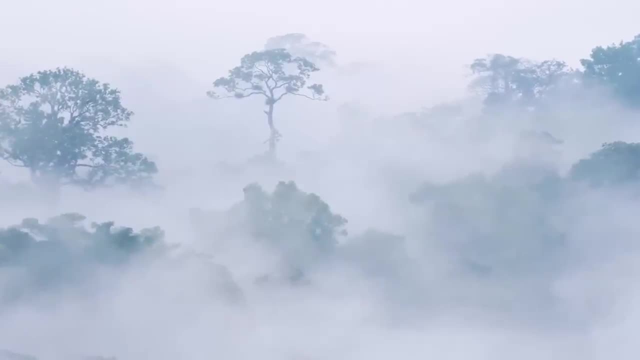 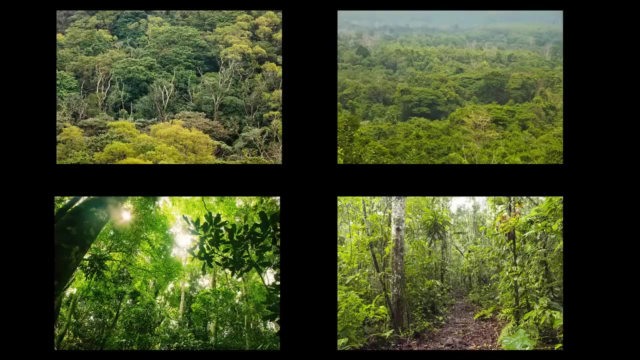 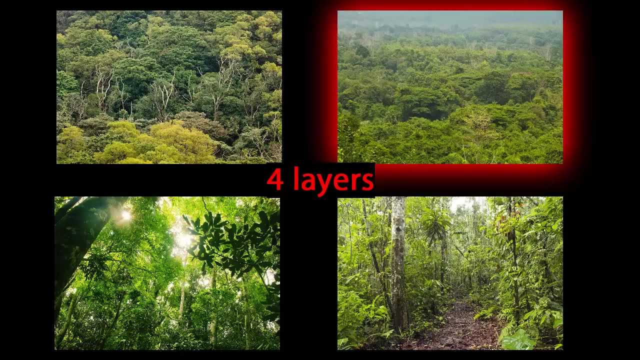 They appear to be wet. They appear to be in the clouds, which is why these areas are called cloud forests. The Amazon, along with every other tropical rainforest, has four layers: The emergent layer, the canopy, the understory and the forest floor. 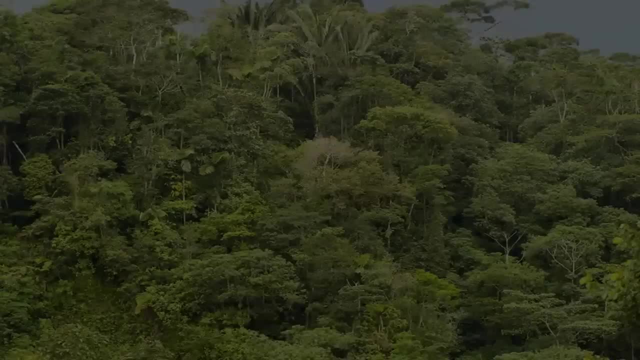 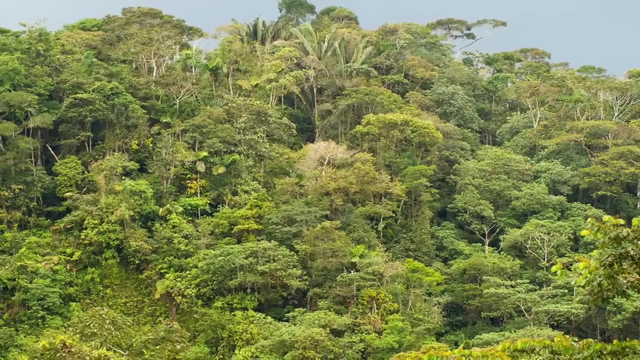 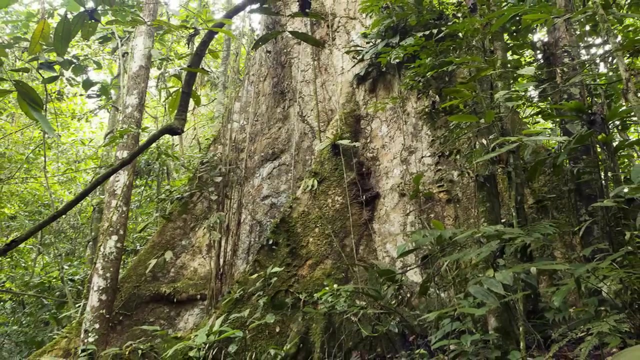 Each layer has its own story to tell. The emergent layer is the highest in the rainforest. It is where the tallest of the trees stick out from the top of the canopy. These are also the oldest trees in the Amazon rainforest, maybe even hundreds of years old. 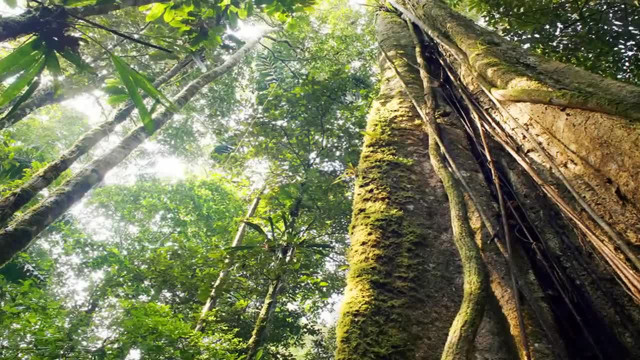 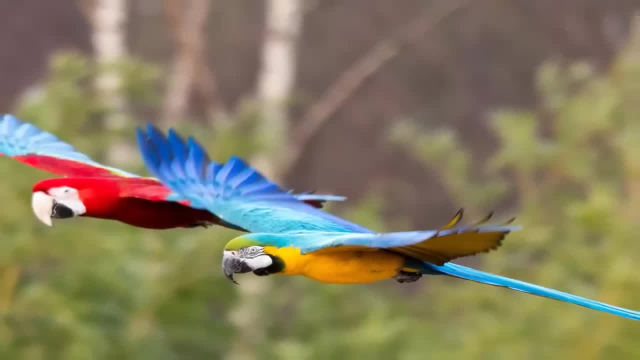 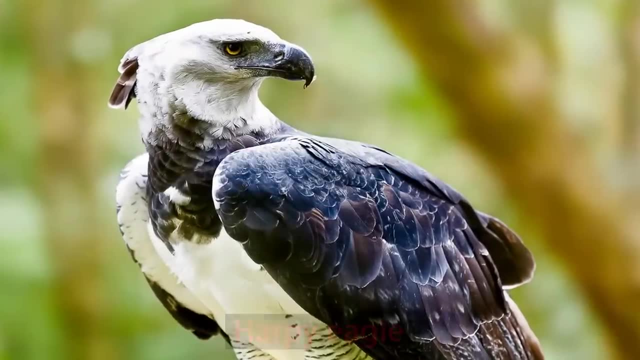 They can easily grow 165 feet tall. Some grow even higher. In order to live so high up in the rainforest, animals need to be able to fly or climb Up this high. you might find the South American harpy eagle using the trees to look for its next meal. 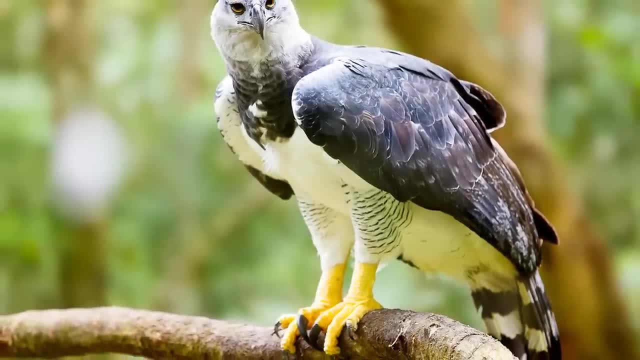 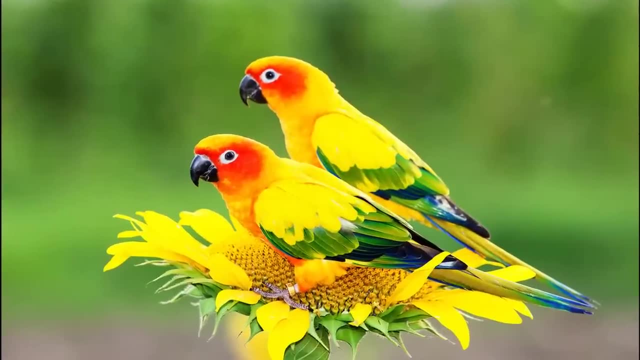 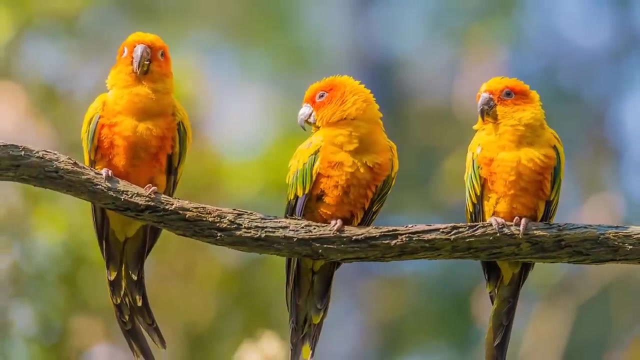 They also protect their young by building their nests up high in the emergent layers. You can see many colorful birds here, including many members of the parrot family. like these conures, These parrots live in noisy flocks high up in the trees. 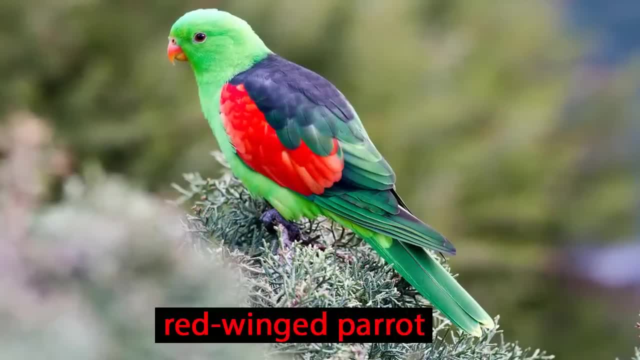 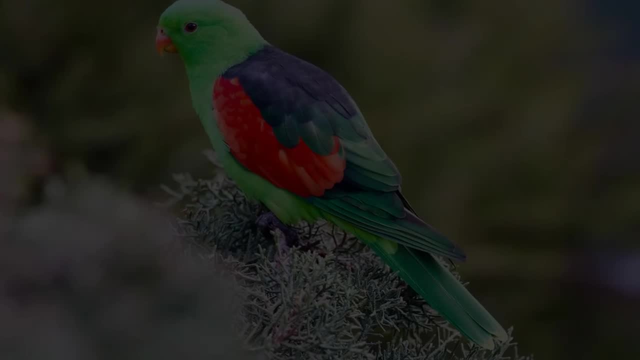 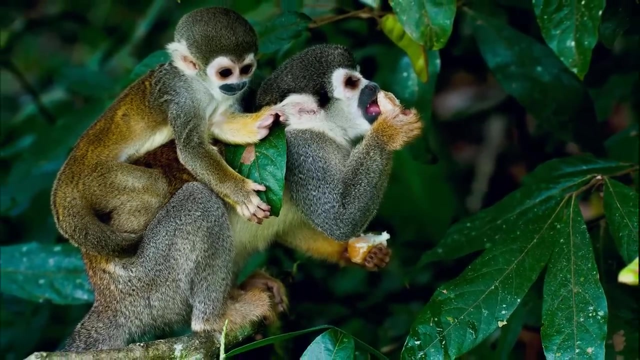 This red-winged parrot uses its strong, curved beak to feed on fruit seeds, flower buds and insects. Spider monkeys can spend their lives up here in the treetops and are expert climbers. They are able to use their arms, legs and even their tail to grip the branches. 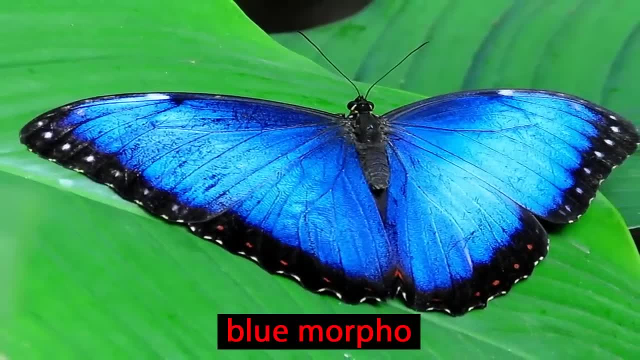 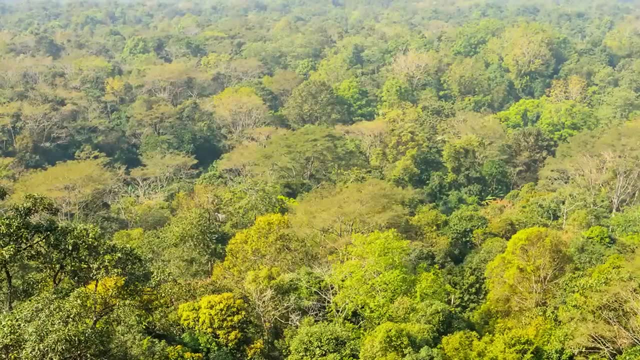 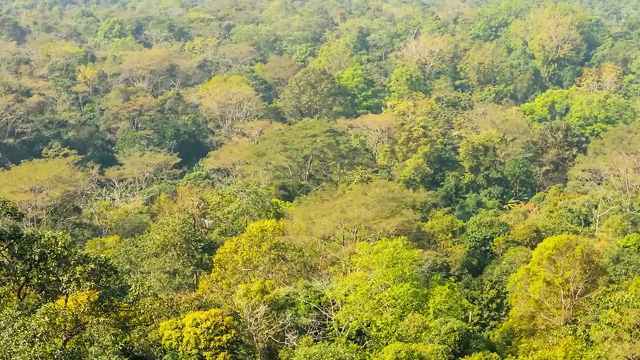 The blue morpho butterfly is one of the many colorful butterflies in the world. You can see many colorful butterflies that we see flitting around the treetops. Moving down to the next layer, we find ourselves in the canopy. This is the umbrella of treetops covering the rainforest. 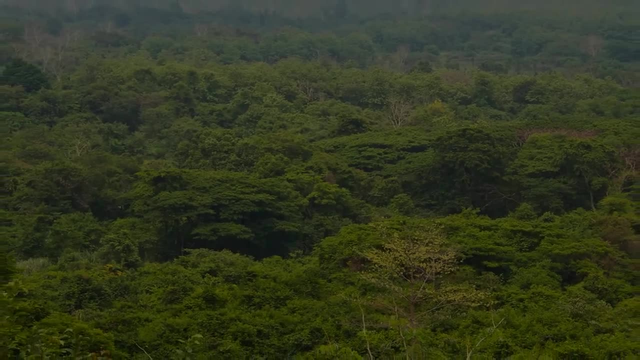 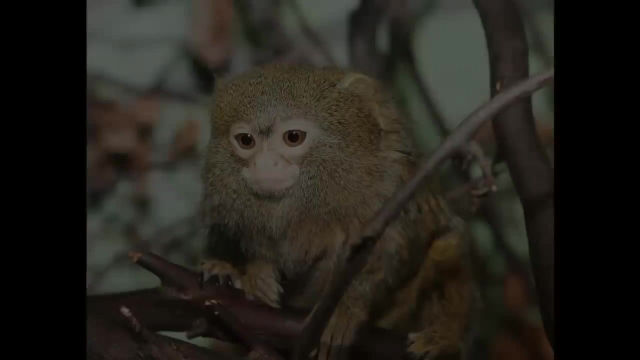 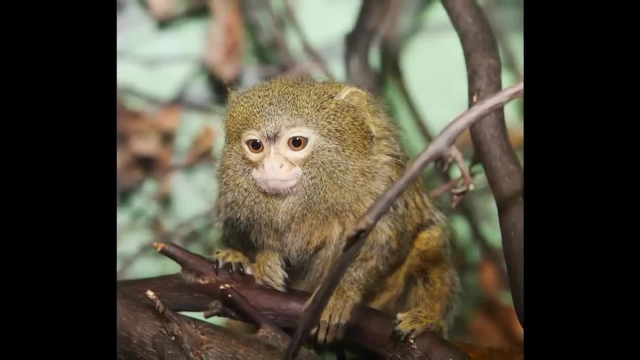 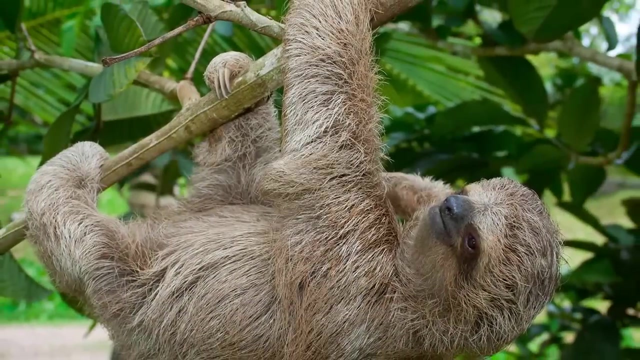 It is the main layer of the rainforest. More animals live in the canopy than anywhere else in the Amazon jungle. In fact, about two-thirds of the rainforest animals live in the canopy. Here you might see this slow-moving sloth who hangs upside down all day, even to sleep. 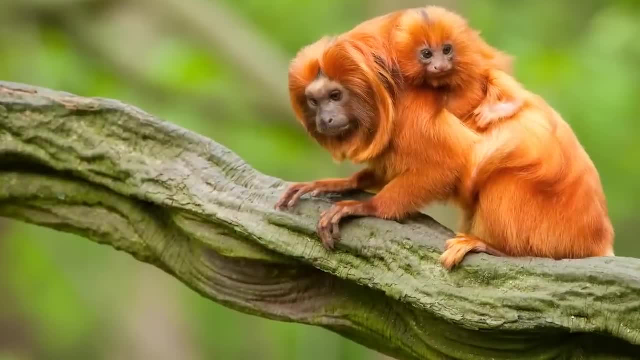 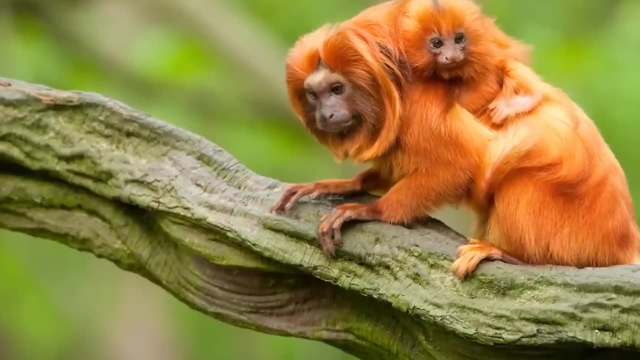 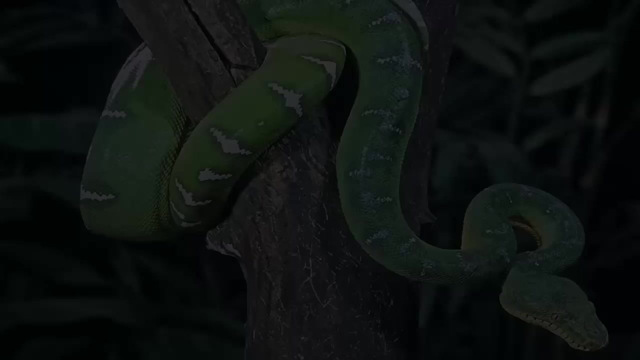 The emergent layer and the canopy share a lot of the same residents: birds, monkeys, snakes, butterflies and insects. You might find this emerald tree boa, another superb climber. See how well camouflaged it is to look, just like the leaves on the trees. 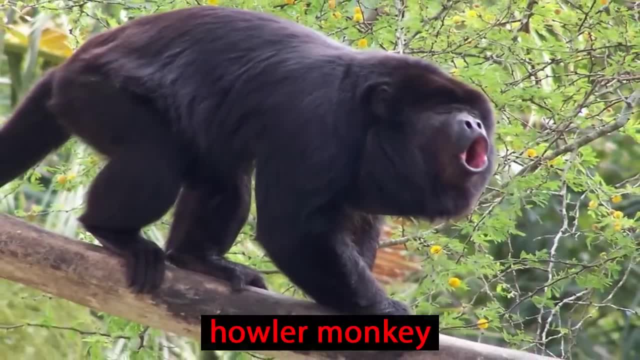 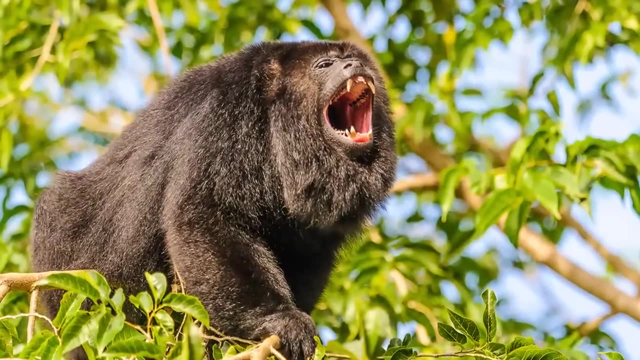 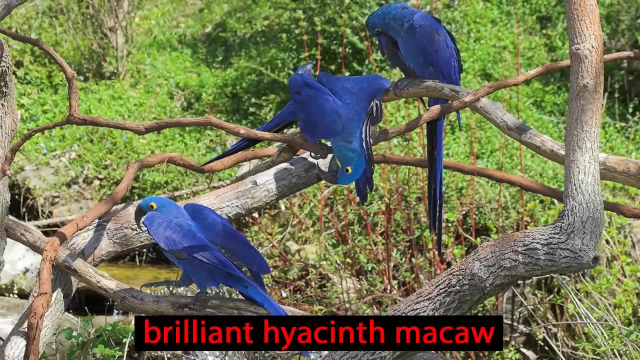 If a heller monkey catches sight of one of these snakes, it will sound an alarm that would be impossible to ignore. The shrieks are ear-splitting. Macaws like this brilliant hyacinth macaw are one of the many birds moving around the canopy. 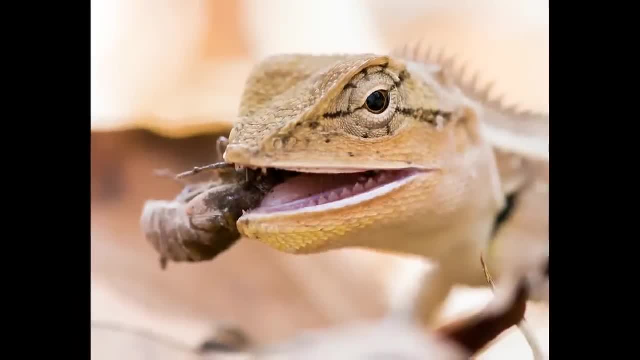 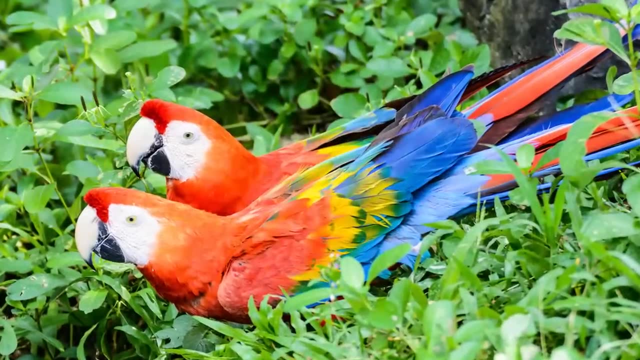 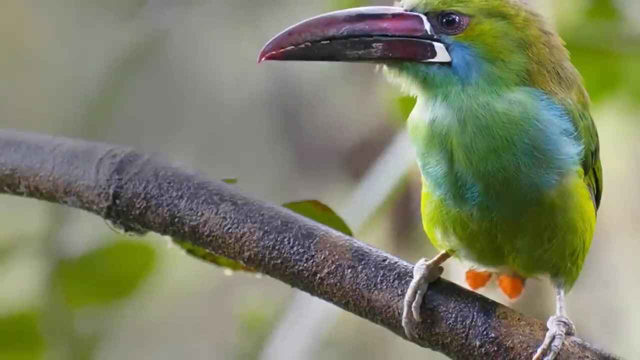 Many animals are able to find food, water and shelter here, and so they have no need to leave. The canopy is the home of choice for 30% of the world's birds, like this red-green macaw, Here is a toucanette. 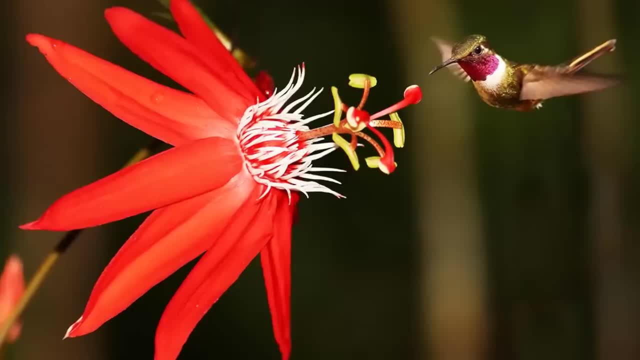 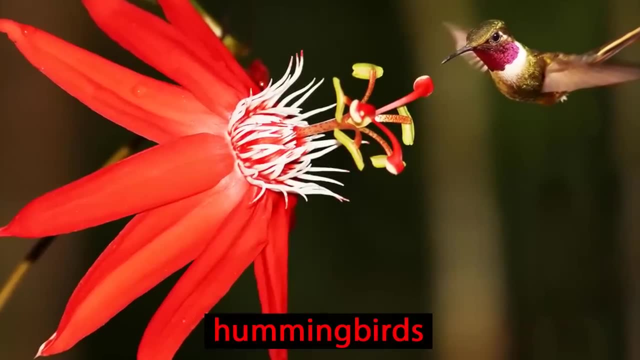 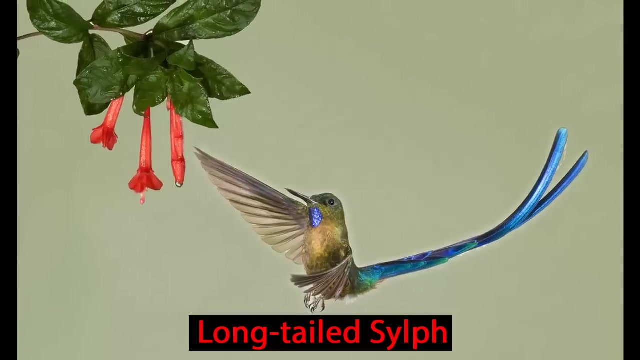 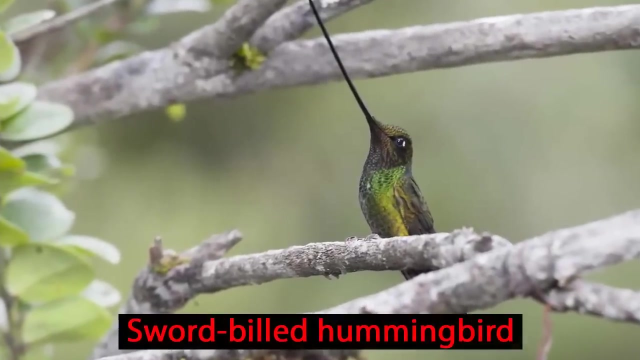 Bird life ranges from giant eagles weighing up to 17 pounds to these tiny hummingbirds weighing only a few ounces. Hummingbirds feed on the nectar of flowers like this long-tailed silk. Beautiful, isn't it Their long bills. let them get deep into the flower, like this sword-billed hummingbird. 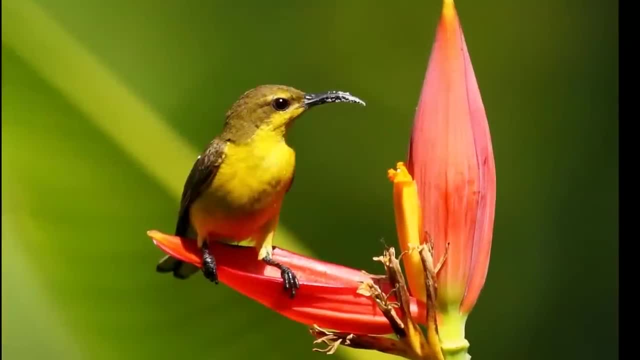 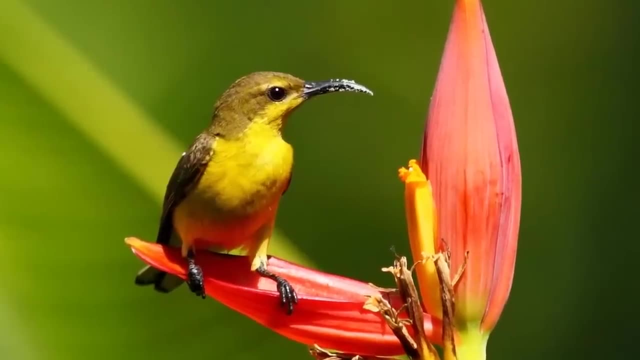 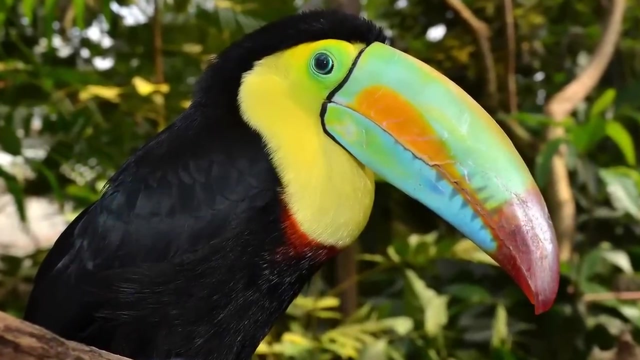 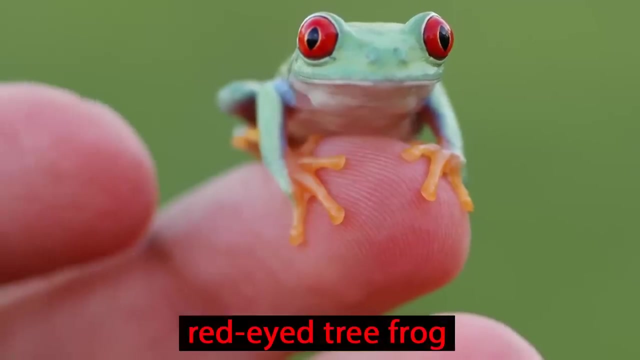 As they feed, they are dusted with the flower's pollen. When they fly away, they spread the pollen wherever they go. These colorful toucans like to hang around the canopy. They eat leaves, fruits and nuts. Here is one of the most recognizable creatures in the Amazon: the red-eyed tree frog. 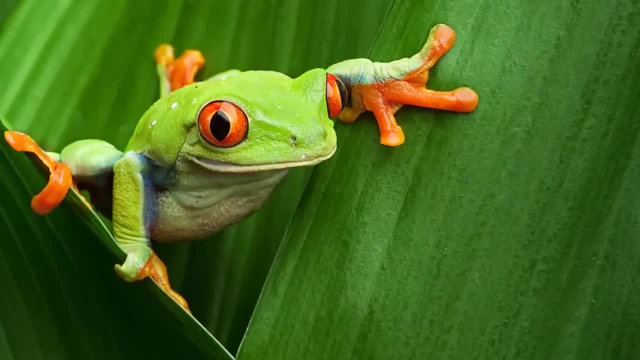 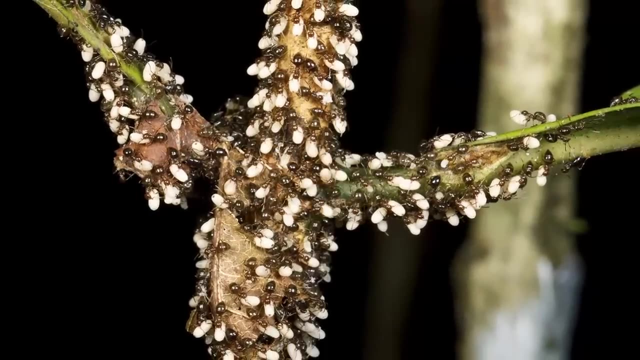 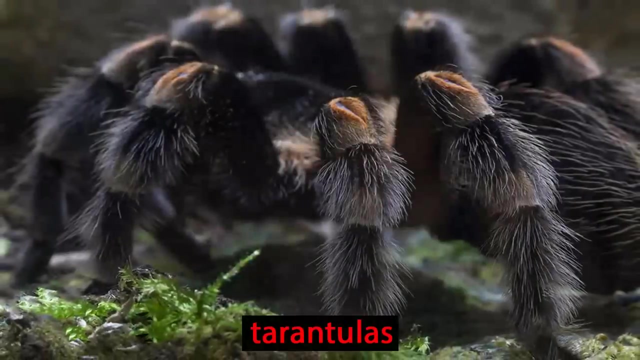 It has suction cups on its tiny feet, allowing it to hang on tight. Insects have an easier time of it, since they can crawl up and down the trees. So can the spiders. These tarantulas are some of the world's most beautiful birds. 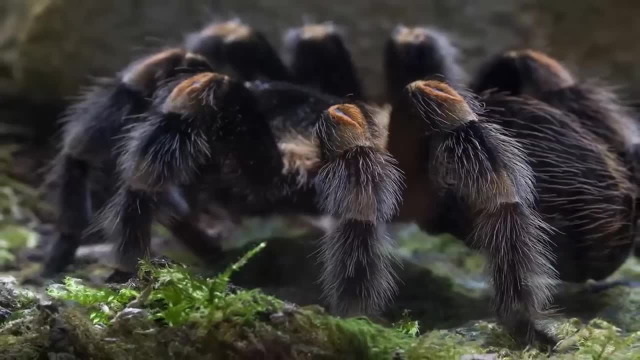 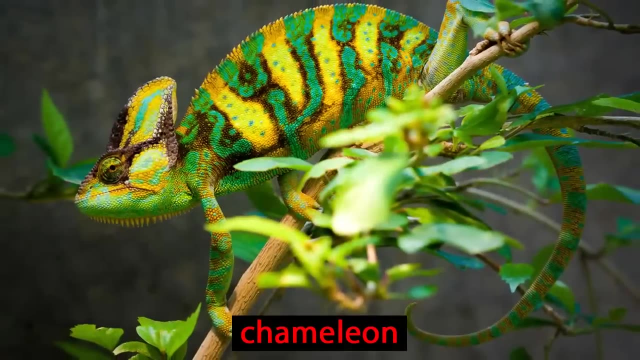 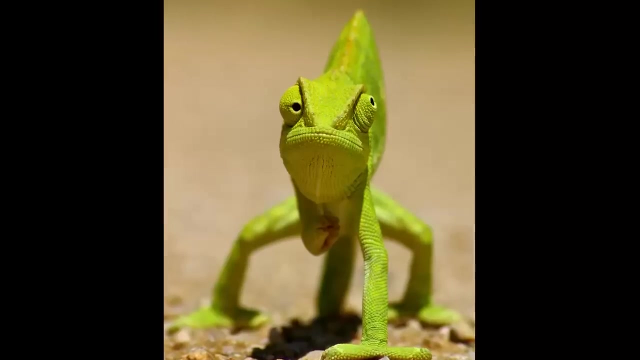 They are as large as spiders and can grow as large as dinner plates. They come out at night to hunt. Chameleons live in the canopy along with other lizards. A close-up look at chameleons show us that they can move each eye separately. 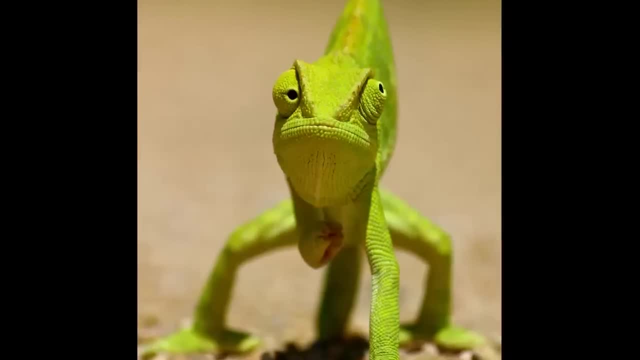 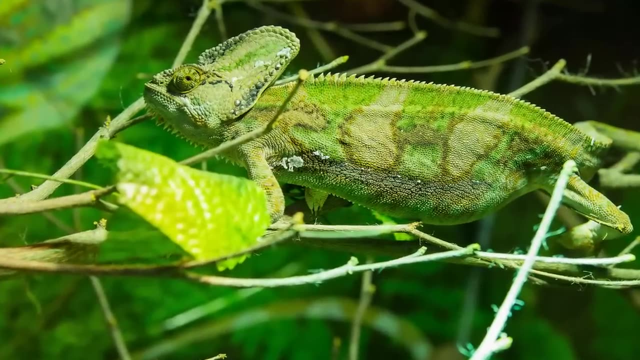 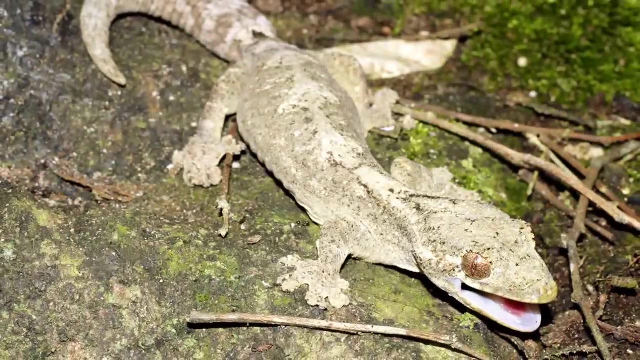 This helps them to be on alert against lurking predators. Chameleons are masters of disguise, Able to change their color if they are scared or if they want to blend into the background. Geckos, too, can change the color of their skin for protection. 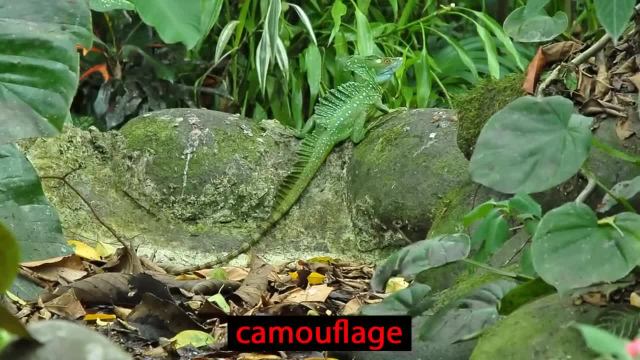 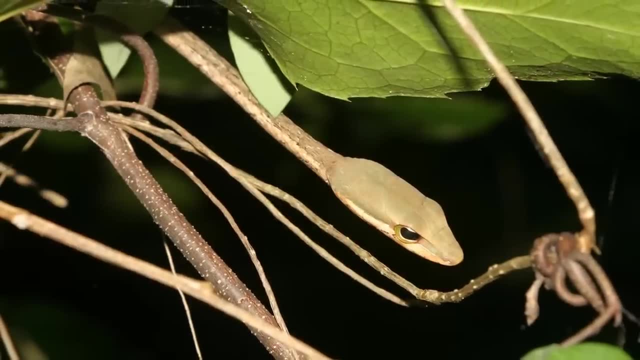 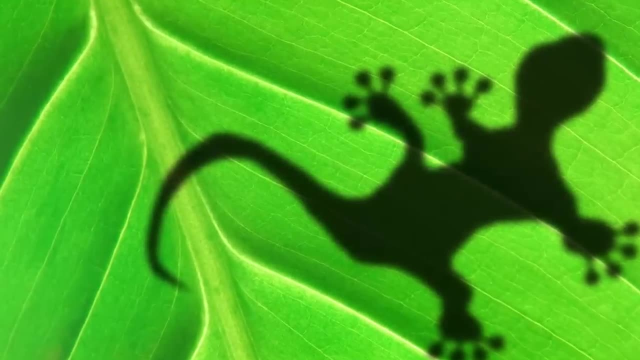 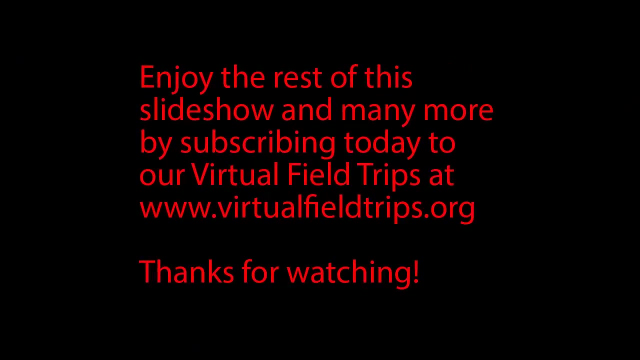 This ability, known as camouflage, helps them to survive. Camouflage allows an animal to either hide from predators or to sneak up on prey when hunting. We hope you enjoyed meeting some of the exciting animals that live in the Amazon Rainforest. To learn more about the Amazon Rainforest, please visit the Amazon Rainforest website.